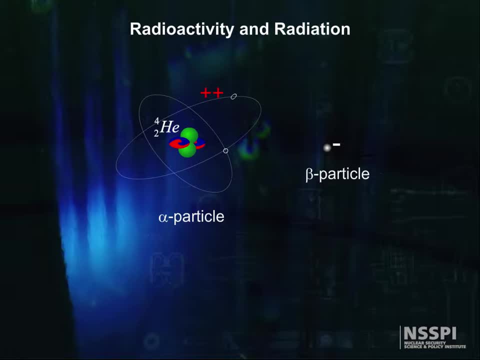 Now that we're done with the naming of the part, let's look at closer at the different types of radiation and their characteristics. Alpha and beta radiation are particulate radiations and are directly ionizing. They lose their kinetic energy by interaction of their charge with the charge of the atoms in the media that they are traversing. 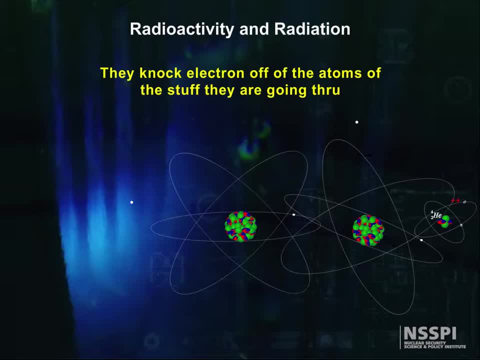 Meaning that the combination of their kinetic energy between the atoms and the media that they are traversing. meaning that the combination of their kinetic energy between the atoms and the media that they are traversing energy and charge. they are able to knock electrons off of atoms, of this stuff. 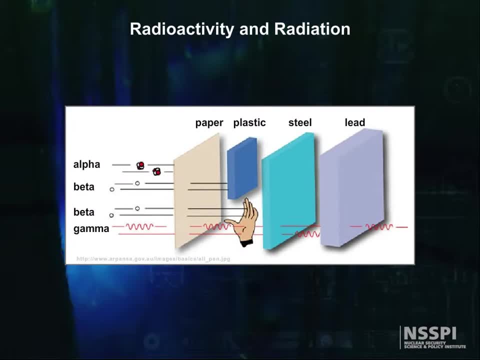 they're going through. both alpha and beta particles have ranges, that is, there are distances that they travel the range and then they are completely stopped. these ranges depend mostly on the type of particle, where there's an alpha or beta, the kinetic energy of the particle and the density of the medium alpha. 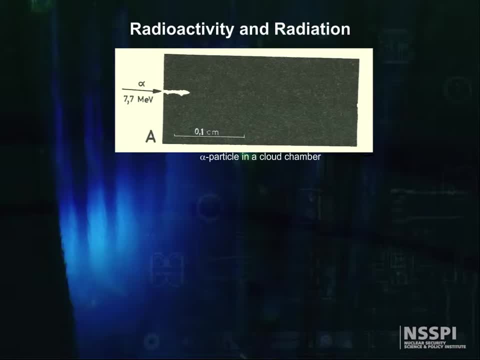 particles are the Tyrannosaurus rex of nuclear radiation. they are huge, they are highly ionized and they beat up whatever they go through. because alphas are so highly ionizing they lose their kinetic energy very quickly. even alpha particles with seven or eight MeV of kinetic energy only travel a few. 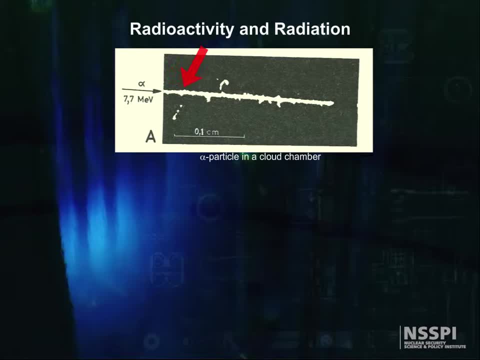 centimeters in air. let's look at an alpha track in the cloud chamber. note the scale at the bottom of the graph and the number of particles that are in the bottom of the figure. the length of the line is one millimeter. there is a central core that is highly ionized and every now and then there is a large 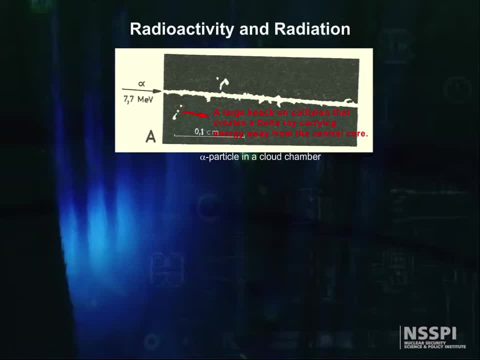 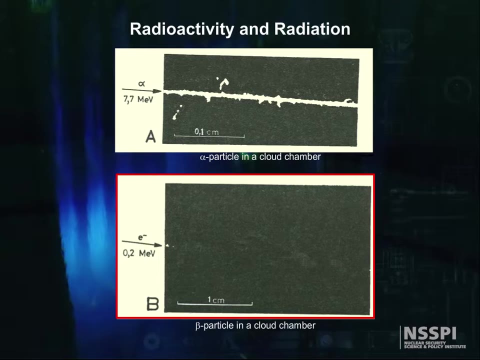 knock-on collision that creates a Delta ray carrying energy away from the central core. for low Z materials, about half the energy is deposited in the central core and about half is deposited by Delta rays, beta particles or electrons, or anti electrons, that are ejected from the nucleus. beta rays are much less densely ionizing than alpha particles and 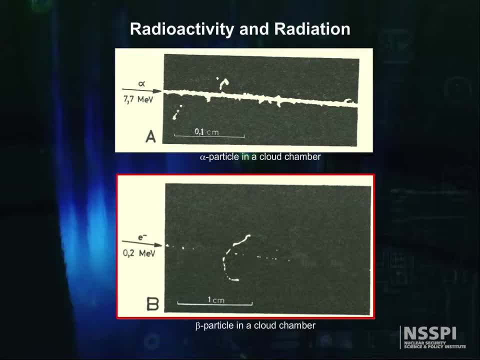 therefore, their range is greater than for alpha particles if they have the same energy. the range of a beta particle in air is about four meters per MeV of kinetic energy. let's look at an electron track in a cloud chamber. notice the scale at the bottom of the figure. the length of the line is now one. 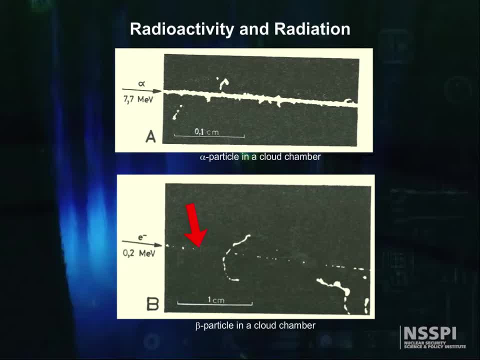 centimeter we see here. during the high energy part of its travel, the electron often travels more or less in the straight line, but near the end of the track, when its kinetic energy is low, it's bounced around much more and loses much more energy per unit travel. the next figure. 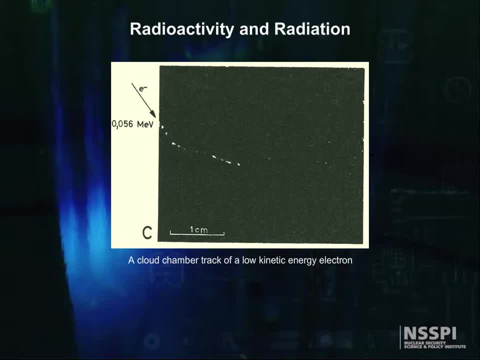 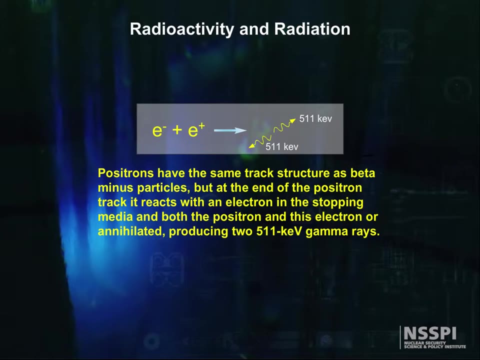 is a cloud chamber track of a low kinetic energy or electron, or, if you will, the track of a high energy electron near the end of its range, where it's lost most of its kinetic energy. positrons have the same track structure as beta minus particles, but at the end. 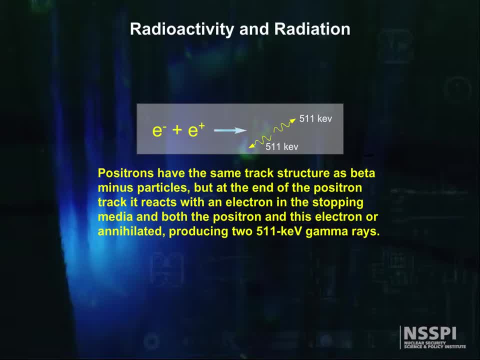 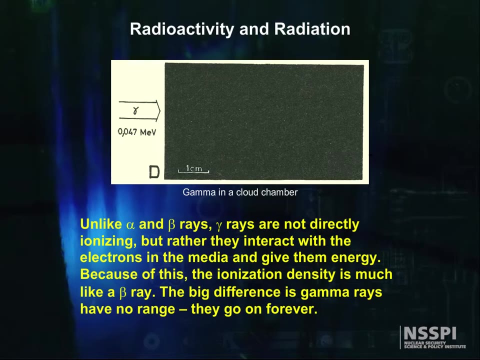 of the positron track. it reacts with an electron in the stopping media and both the positron and this electron are annihilated, producing two 511 keV gamma rays, speaking of gamma's. unlike alpha and beta rays, gamma rays are not directly ionizing, but rather they interact with the electrons in the media and give them energy. 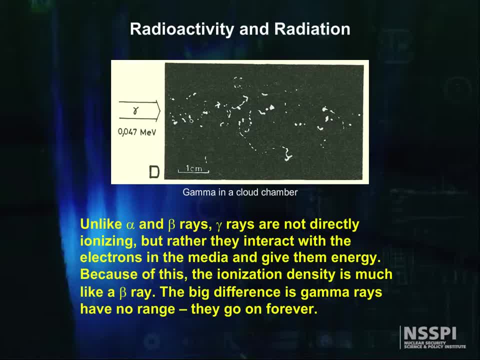 Because of this, the ionization density is much like a beta ray. The big difference is gamma rays have no range. They go on forever. They do have half-value layers, however. By using shielding we can lower the dose from gammas to whatever level we want, except zero. 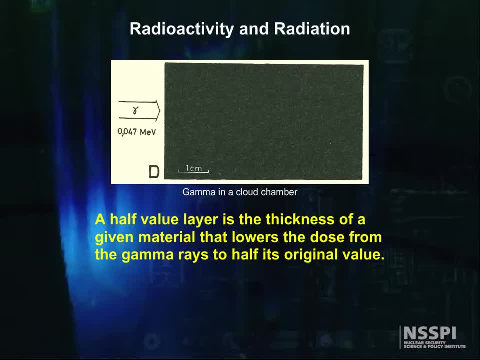 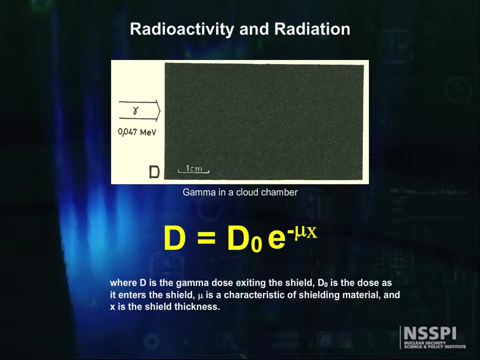 A half-value layer is the thickness of a given material that lowers the dose from gamma rays to half its original value. Guess what two half-value layers do. In math, D equals D-naught E to the minus mu-x, where D is the gamma dose exiting the shield. 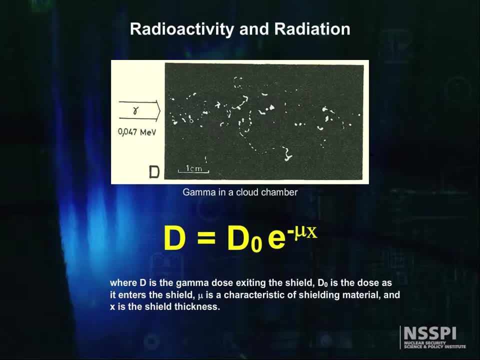 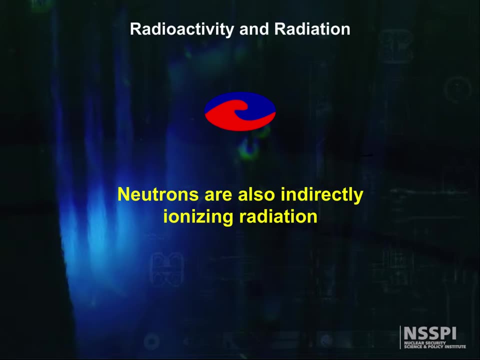 D-naught is the dose from the gammas as it enters the shield. mu is a characteristic of the shielding material and x is the shield thickness. There's a reason. this looks very much like the half-life decay equations. Finally, neutrons are also indirectly ionizing radiation.